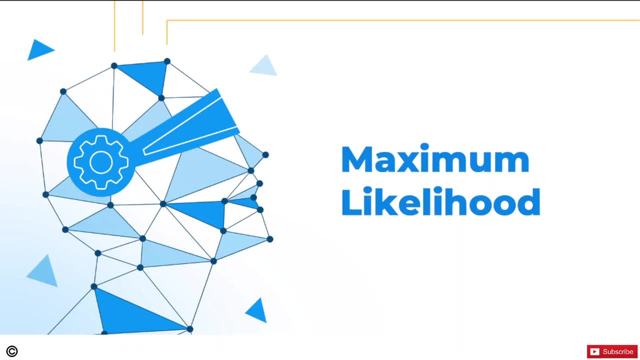 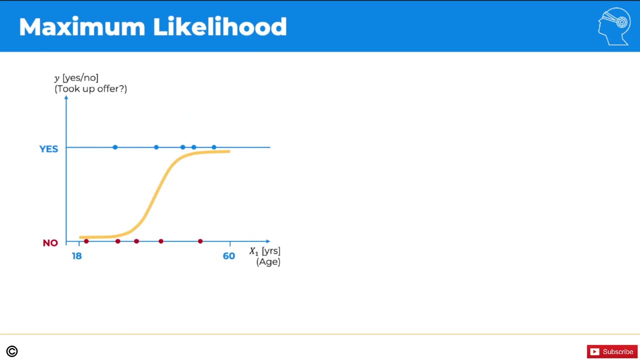 Hello and welcome back to the course. Today we're talking about maximum likelihood. So we have this curve that's fitting our data. It's great. but how do we know that this is the best curve that can fit our data? Just like with linear regression, there could be multiple curves of this shape that 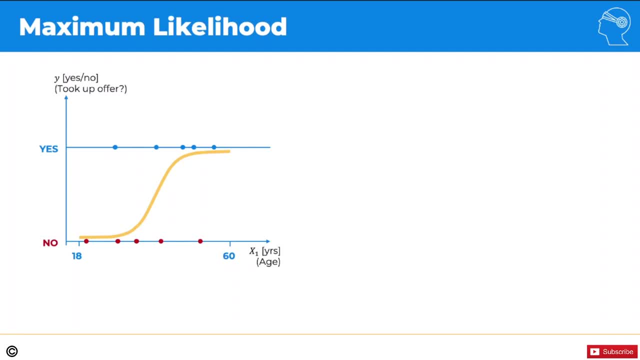 could fit our data. So how do we find out which one is the best one? Well, we need to calculate the maximum likelihood, And the way it's done is by looking at each data point. So, for example, we start here and finding out for the person of that age what would have this curve that we're 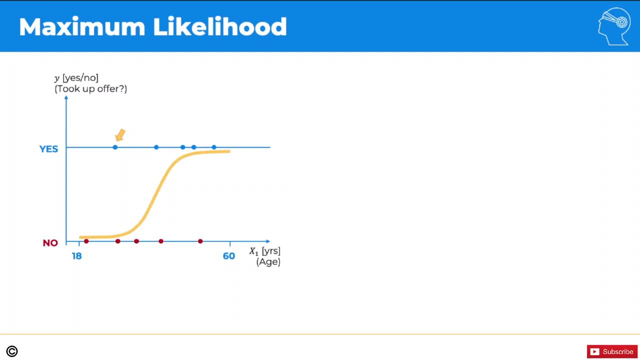 potentially considering. what prediction would it have made? So this specific curve, this specific logistic regression that we've modeled, it would have said that a person of that age has only a three percent chance of saying yes or taking up the offer. So it's a. 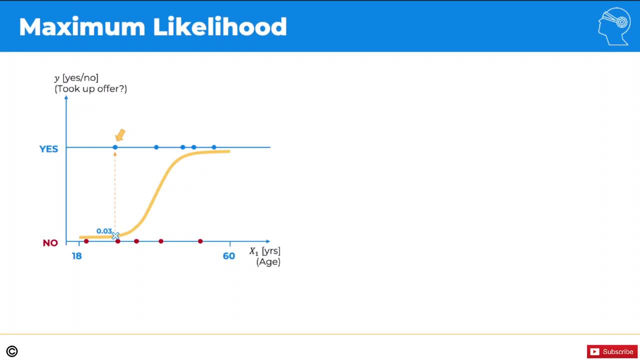 very low probability. And then it's a very low probability that a person of that age will have a three percent chance to say yes or taking up the offer. So it's a very low probability And low chance for this person or this person of this age to take up the offer. And then we would 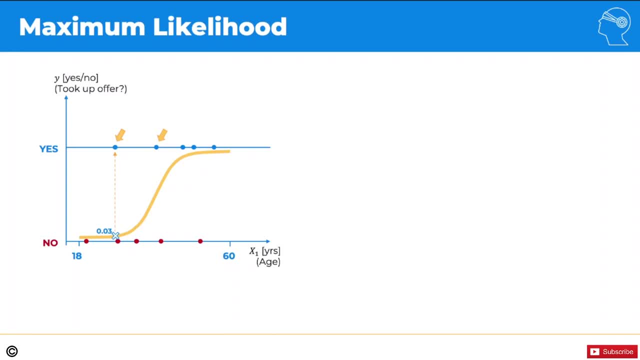 continue. So for the next point, what would have the logistic regression modeled? So we know that this person took up the offer, We know it's a yes, because that's our input data, But what would have the logistic regression said if we didn't know that the person took up the offer And the 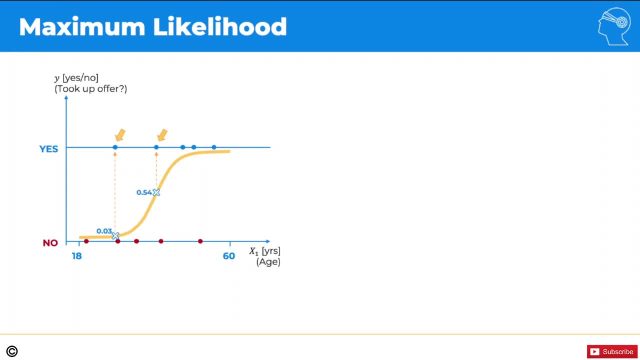 logistic regression, the point would be somewhere here on the curve and that would be 54%. chance for this person or for this data point would be 92%. For this data point: 95% For this data point, our logistic regression for that specific age, a person of that age, predicts 98%. So we've got all. 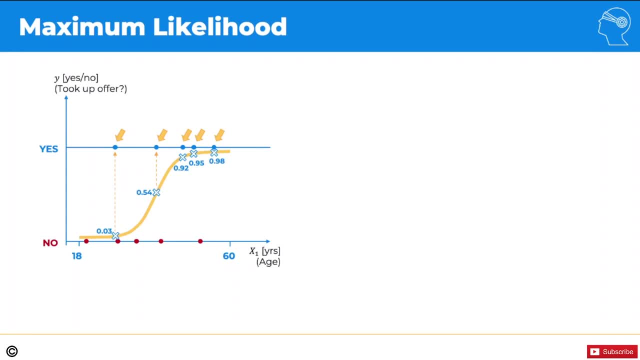 those numbers Great. Now just to make, to avoid cluttering this image, we'll do the bottom points on a separate image. So for this point, the logistic regression predicts 1% chance. for this point, for somebody of that age, the logistic regression predicts a 4% chance.